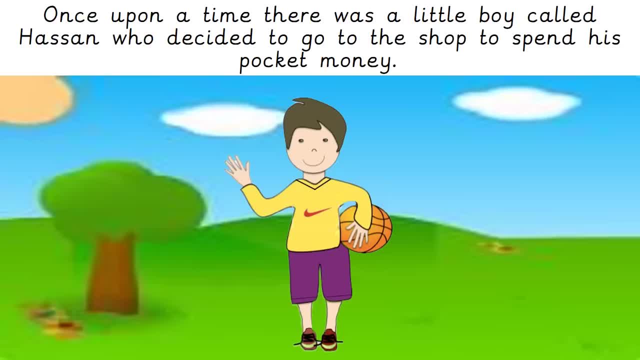 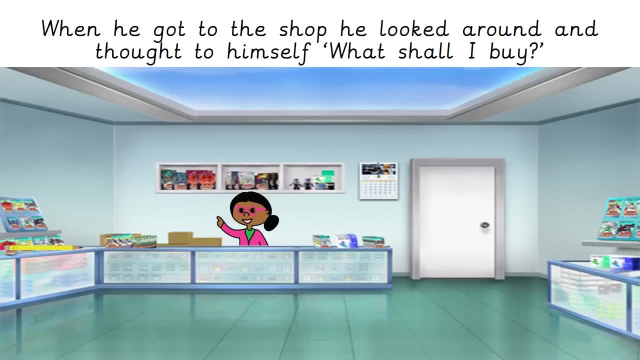 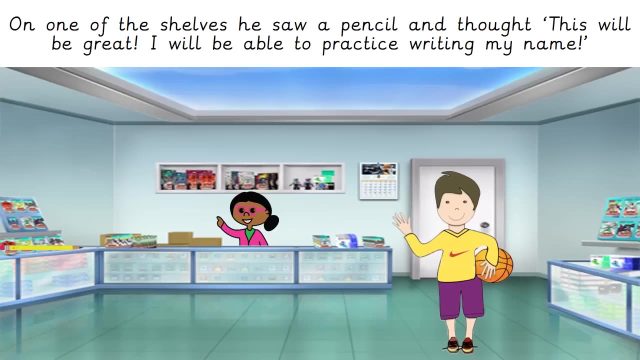 Once upon a time there was a little boy called Hassan who decided to go to the shop to spend his pocket money. When he got to the shop he looked around and thought to himself: what shall I buy? On one of the shelves he saw a pencil and thought: this will be great, I will be able to practice writing my name. 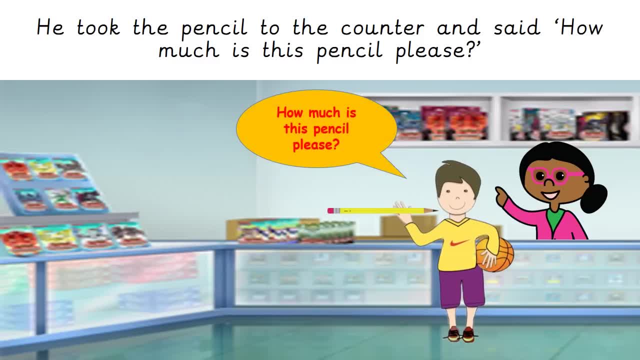 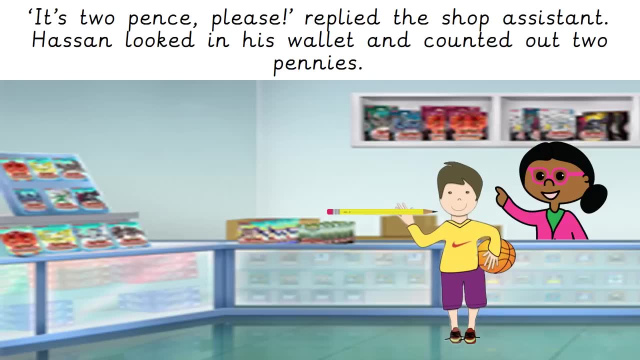 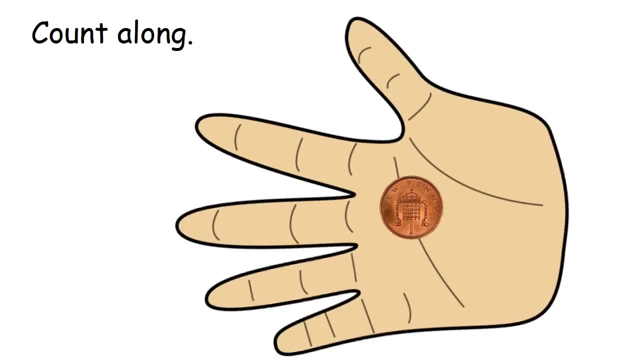 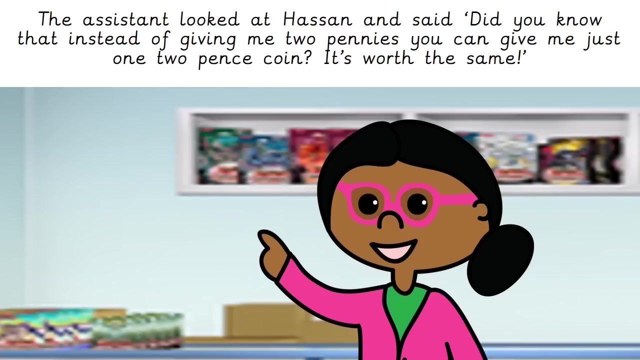 He took the pencil to the counter and said: how much is this pencil, please? It's two pence, please, replied the shop assistant. Hassan looked in his wallet and counted out two pennies: One, two. The assistant looked at Hassan and said: did you know that, instead of giving me two pennies, 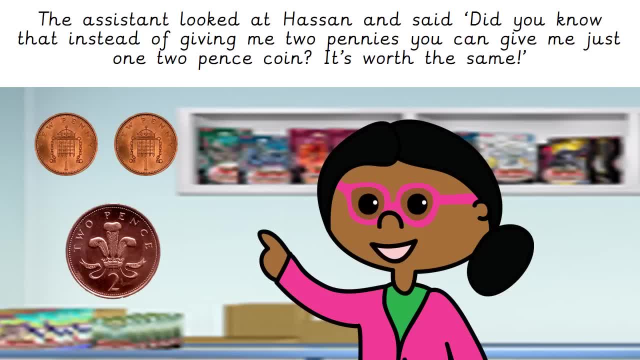 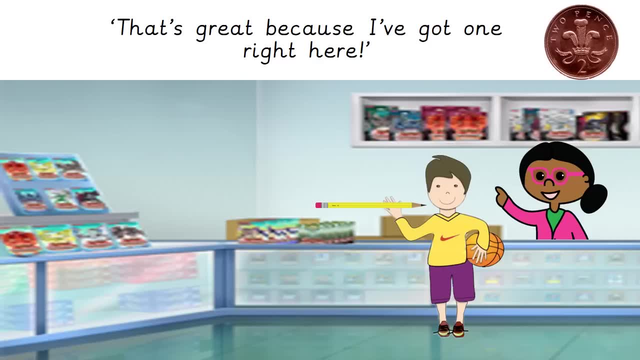 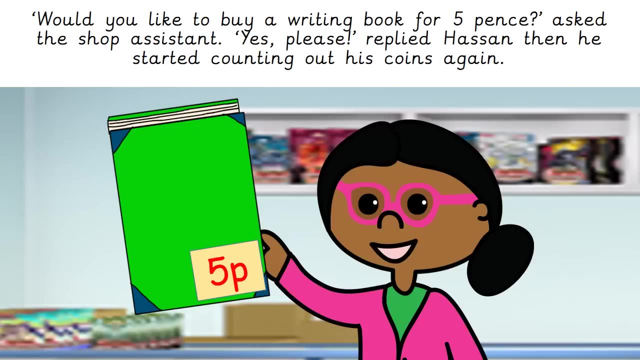 you can give me just one two pence coin. It's worth the same. That's great, because I've got one right here. Would you like to buy a writing book for five pence, asked the shop assistant. Yes, please, replied Hassan. Then he started counting out his coins again. 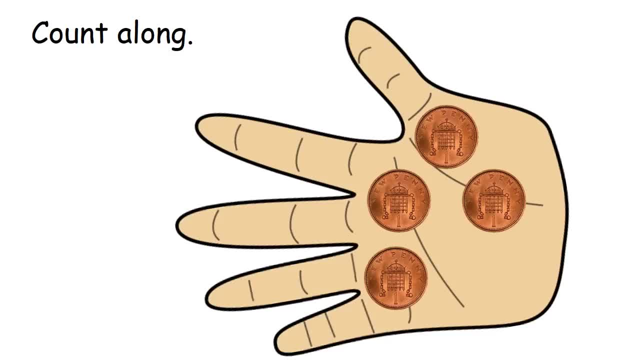 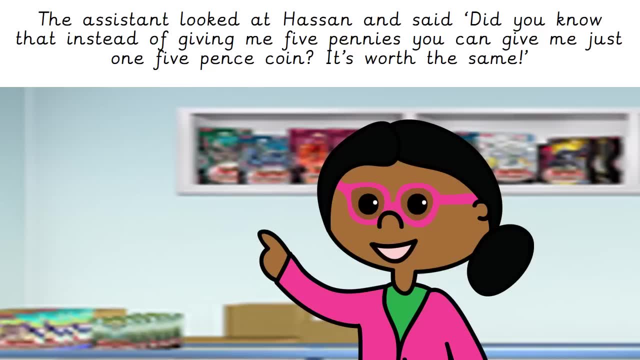 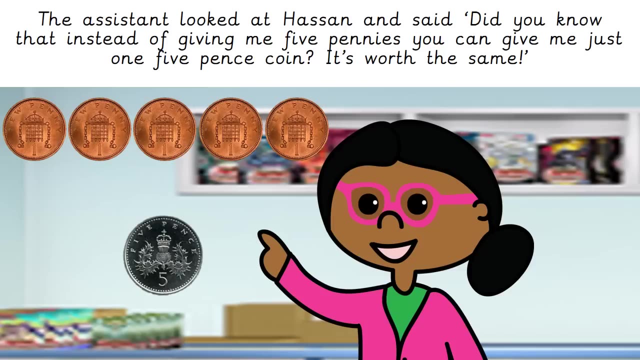 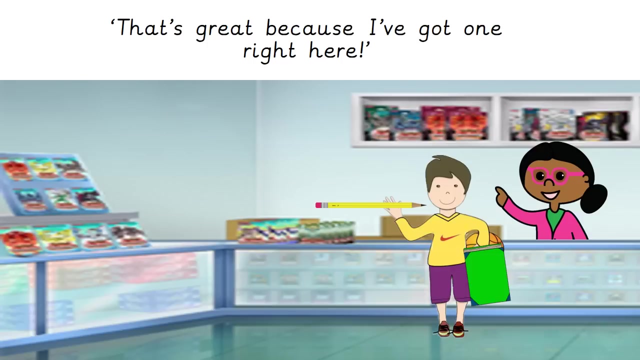 One, two, three, four, five. The assistant looked at Hassan and said: did you know that instead of giving me five pennies, you can give me just one five pence coin? It's worth the same. That's great, because I've got one right here. 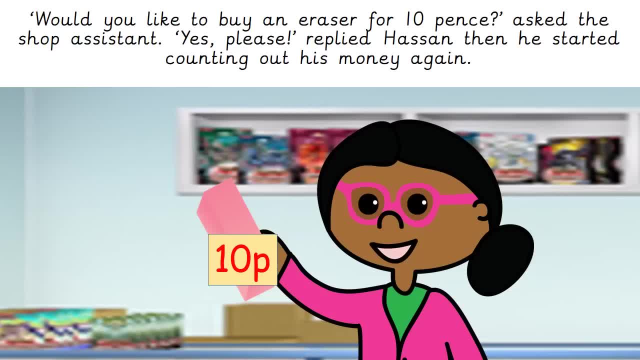 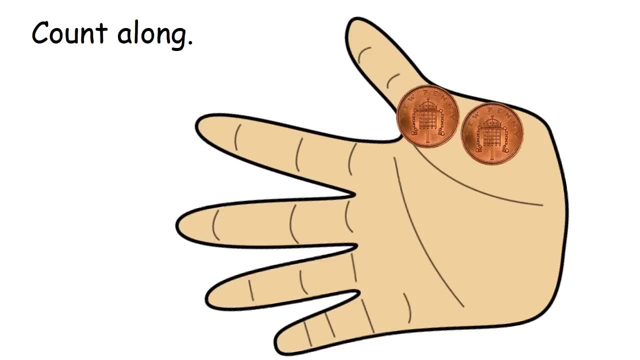 Would you like to buy an eraser for ten pence, asked the shop assistant. Yes, please, replied Hassan. Then he started counting out his coins again: One, two, three, four, five, six, seven, eight, nine, ten.